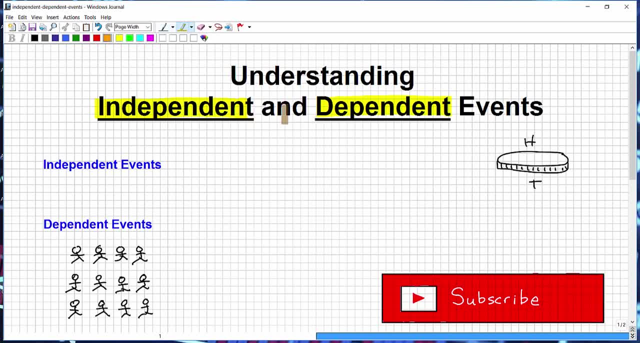 Now the big thing here is that both independent and dependent events are going to be those probability questions that we have, that have the word and in them, Okay. so I'm going to kind of write the rule down. We'll start with independent events first. Okay, I'm gonna write the rule down and we'll explain it. So a probability of A and B occurring is going to be the probability of A and B occurring. 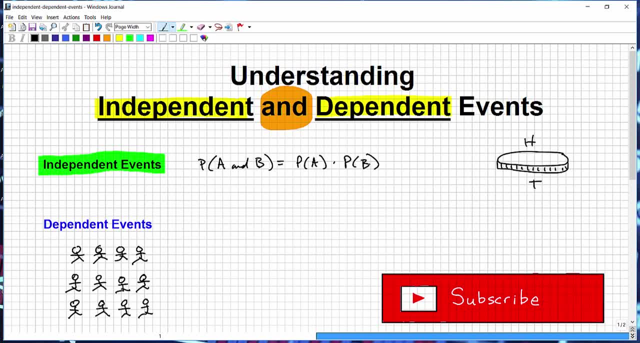 Times the probability of B. Okay, so this is independent events. So let's get into this a little bit more in detail. So let's say I, over here, I have my little. this is a coin, This is what this is supposed to be called. a quarter dime, whatever doesn't make a difference, But this is a coin. Okay. so let's say, I want to know the probability of us, of you getting a tail on a flip and then getting the tail again. Okay, so what's probably getting a tail? and then 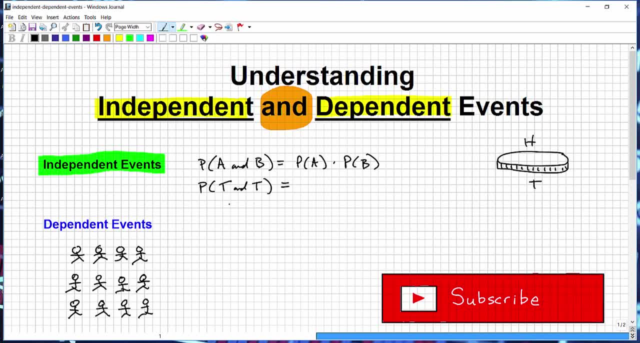 And a tail, Okay, or a head and a head, doesn't make a difference, Okay, but this is this word and is in there. Now, this is the real critical thing that I'm going to really stress to you. Okay, the difference between independent, dependent events. 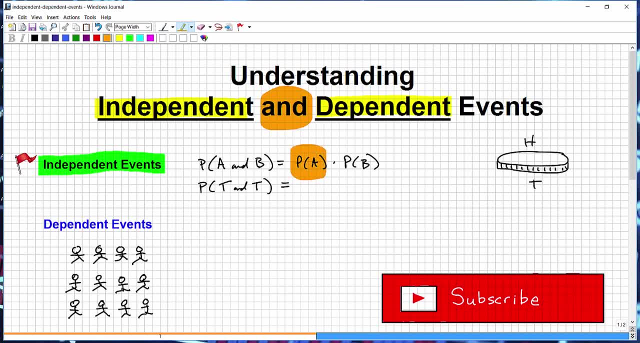 And it's the following: Okay, the probability of A occurring, Okay, is not going to have any influence of the probability of B occurring. In other words, These events that we're looking at Have no bearing on one another. So let's go back to our coin flip here. Let's say I flip this coin and I get tails. Okay, so what was the probability of me getting tails on this? Well, it's going to be a one out of two chance, right, Or 50%. Now, if I got tails on my previous flip and I'm got the coin again and I'm going to flip it again, It is is somehow just because I got tails the last time. Does that increase my chances of getting tails on my current flip? 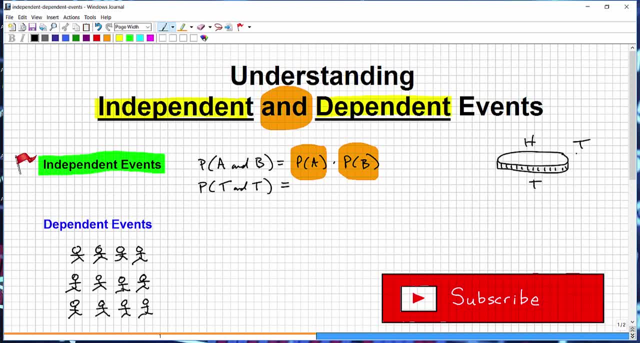 No right, It doesn't. It's not going to have anything to do with it. So this is the key with independent events: The, the what, the probability of something occurring- Okay, like the probability of event A occurring has nothing to do. It's like I have any bearing on the probability of the second thing. Okay, now, this can actually go on and on, But let's just kind of keep it simple. In other words, you can have multiple events, But this is the main idea here. All right, So with independent events, okay, we're talking about the probability of. 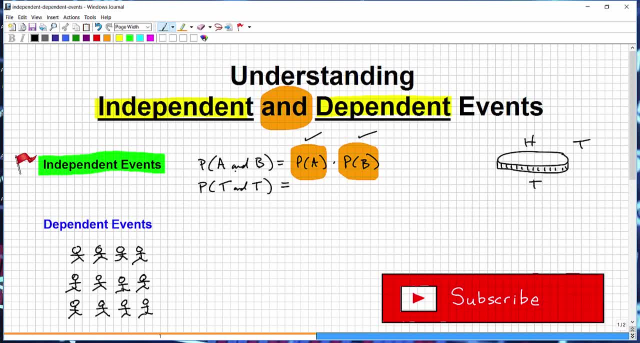 something and something else occurring- Once again stressing the word- and so you can detect that in your probability prompts. So when you're looking at your scenario, ask yourself: is that situation kind of like a coin toss scenario, where one thing's not going to have anything to do with another? Well, if that's the case, then you have independent events. Okay, so this will be the role they're going to be using. All right, let's. 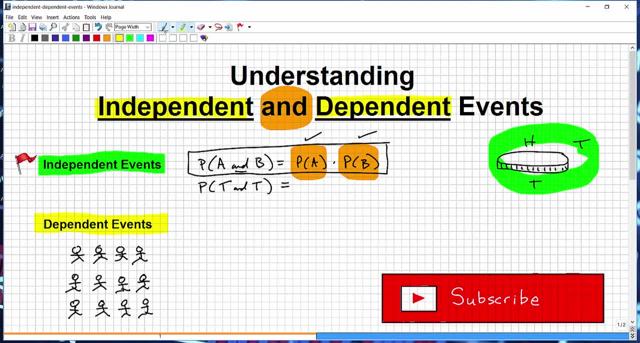 get into dependent events, All right. And this is again the probability of A and B occurring. So same kind of scenario, but this one's a little bit different. I don't think it's more difficult, but it is different. So the rule is it's going to be the probability of A occurring times, the probability of B given. 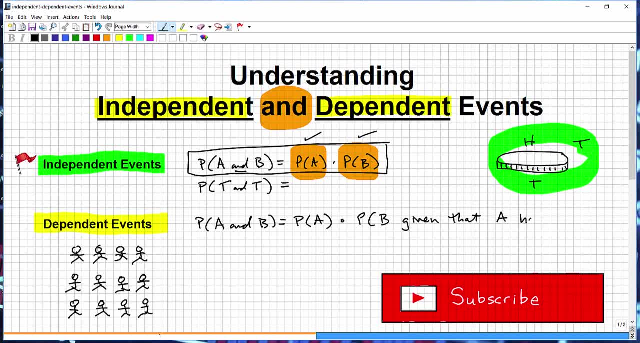 that A has occurred. All right, All right, let me go ahead and give you an example. All right, So, and you can see my little sketch here. Let's say I got a group of students in the classroom And let's see there's four times three, So this is 12 students. Let's say this guy is Sam. Let's say this person over here is Bill, So, and let's say each one of these students has a. 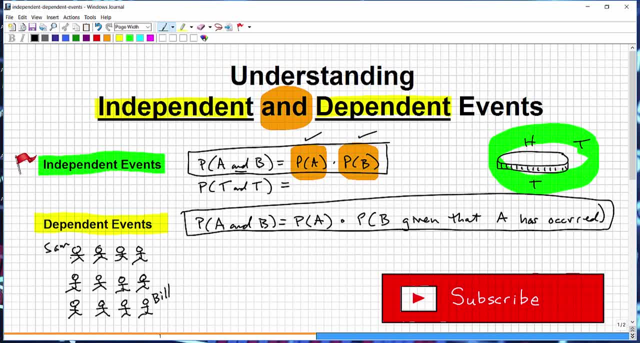 their name, like on a piece of paper, in a jar. Okay, And then teacher is going to be kind of selecting names out of that jar randomly, Okay, so let's try to figure out what's the probability that the teacher selects Sam and then Bill out of that jar. Okay, Sam and Bill, All right. So once again, this is a probability of something and something else occurring, All right. So once again we're looking for that word. 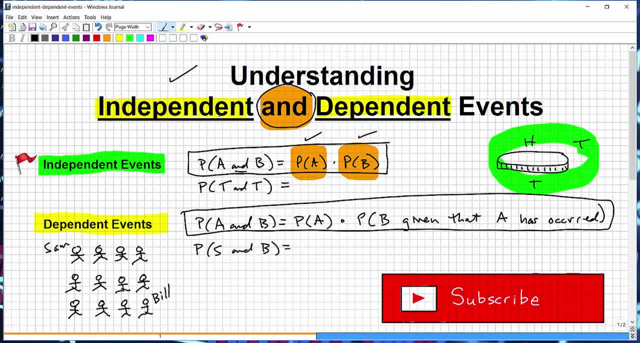 hand, All right. So so far we've already ascertained it's either going to be an independent or dependent events. There are exceptions, but let's kind of keep focused here on these two big concepts and probability, All right, So. so the probability of selecting Sam- okay, if there's 12 students, okay, is going to be what? Well, the probability of Sam being selected is going to be one out of 12.. Right, So let's say the teacher picks. 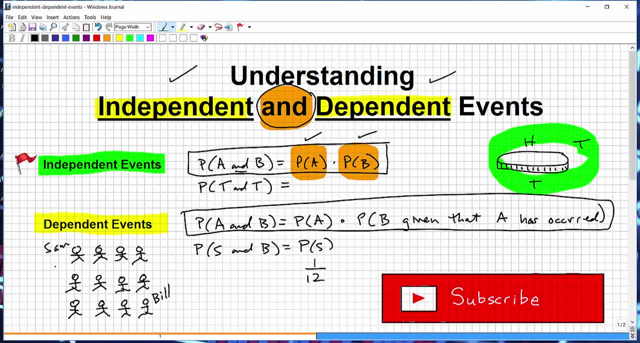 Sam and now she has Sam on, took Sam's name out of the jar And now she's going to go back in and pick another name. Okay, So what's going to be the probability of Bill the second time around she goes to pick? Well, if you think about it, okay, it's going to be different than the probability of Sam. Okay, Sam had a 1 in 12 chance of being selected. Now the probability of Bill being selected is going to be what? 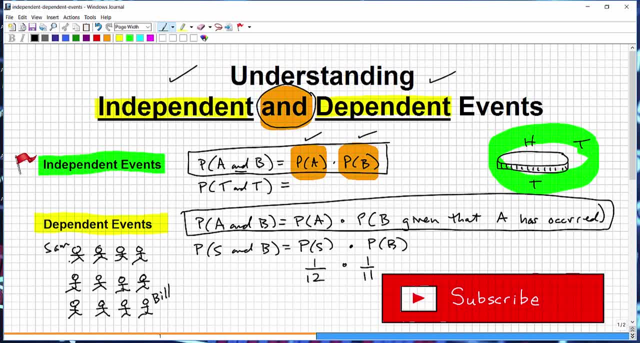 out of 11. all right, because Sam's name is now already out of the jar. all right. so dependent events, all right- is the kind of opposite of where independent, where you have independent events, recall independent events, one thing, the event of one thing had nothing to do with the event of something else, but dependent. 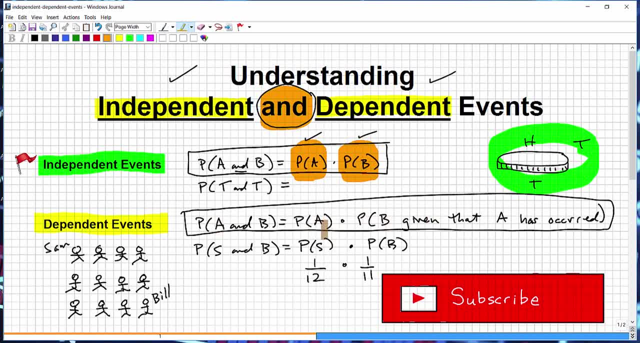 events, they do have influences on one another. okay, so we have to consider if you have a situation where the probability we have to consider the probability of the first thing occurring, that hey it's going to impact the probability of the second thing occurring. all right, if you have that. 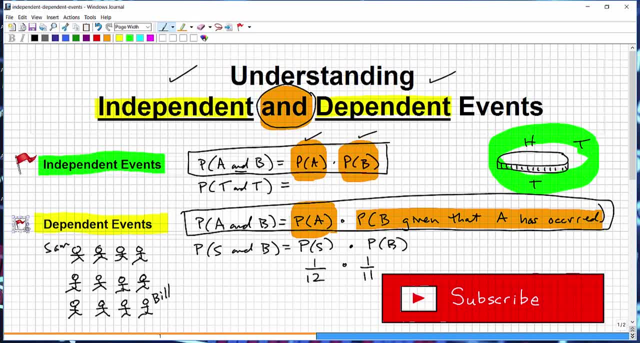 kind of situation. you're going to be dealing with dependent events. okay, dependent events, so big picture, all right. is this: when you're looking at scenarios of the probability of a and B occurring, be thinking independent and dependent events. you're going to be thinking one or two of these scenarios. what you have to do 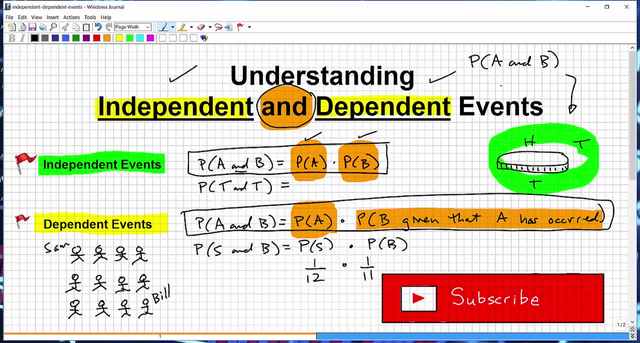 is figure out? is the scenario kind of like the coin tossed? or is it kind of like this example where you have kind of like the students, where one thing is going to affect another thing? okay, by the way, just on the last note, these rules okay can go on and on and on. for example, the probability doesn't have to.